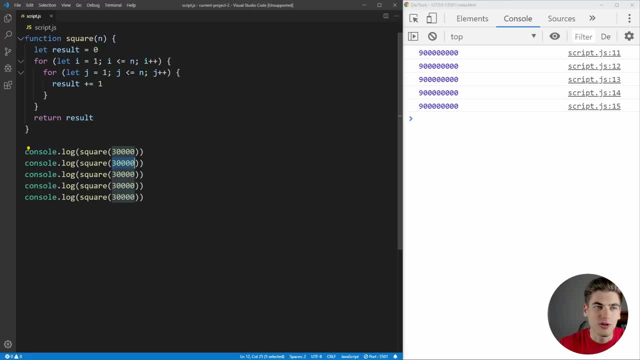 we're caching the value based on the inputs. So in order to do that, all we need to do is create a variable here, and this is going to be for our previous values, and we're just going to set this to an empty array to start. Then what we want to do is after we've calculated: 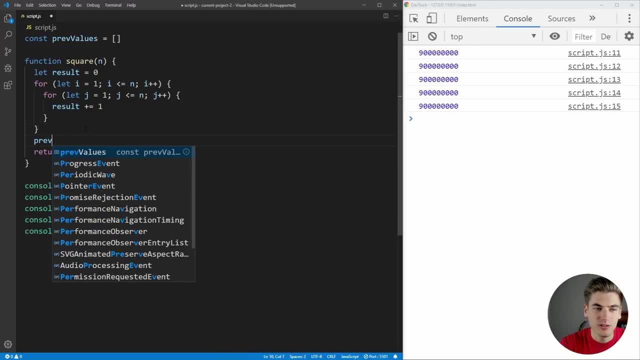 our result. after we've done all of the really hard work. we just want to store that value instead of our previous values, just like this, So we can say result. So essentially every single time we call this function, we're going to store the result in the nth position. 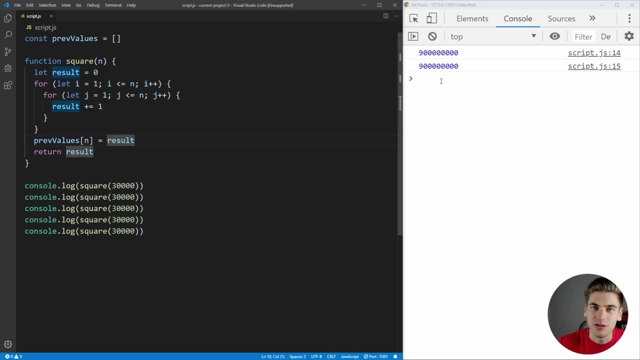 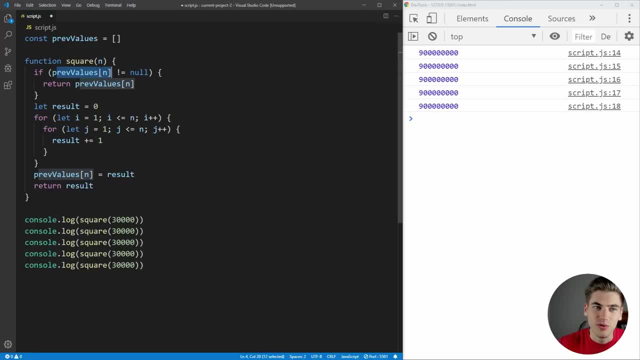 going to save this, And then we're going to save this, And then we're going to save this. So this is saying: if we've already called this function with this variable n, just return the results since we saved it down here. Now, if I run this, you can see the first one execute slowly, but 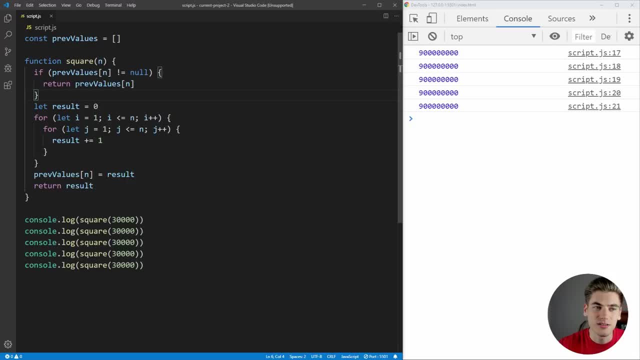 every single other one finishes instantaneously, because all it does is look up the value that already exists. Memoization is used literally everywhere inside of programming, And some really popular use cases are this: where you have a really slow function that takes a long time to execute. 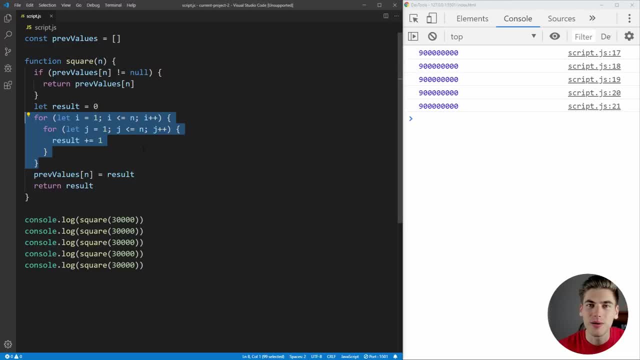 and you want to get the same value over and over. Another really popular use case is when you're fetching external resources, So you're using the fetch API. then using memoization will save you from having to make a bunch of calls to the server. 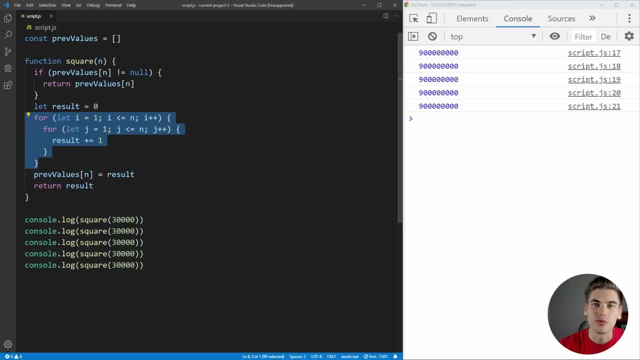 because you already know if you've made that call and you already know what the results are. you've essentially cached them. The last major use case of memoization is in dynamic programming, And dynamic programming is when you take a recursive function that calls itself multiple. 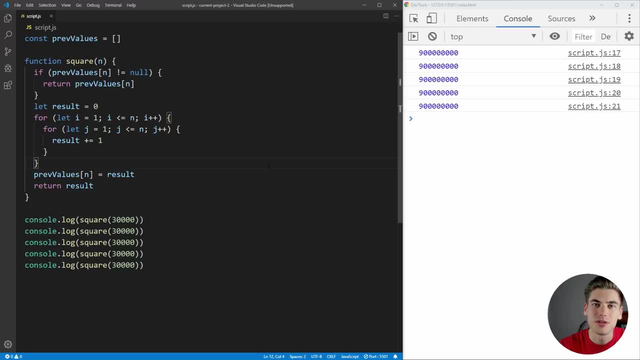 times with the same inputs and you actually memorize those inputs. So if you're not familiar with recursive functions, I have an entire video on them linked in the cards and the description below. you can check out. But to get started, 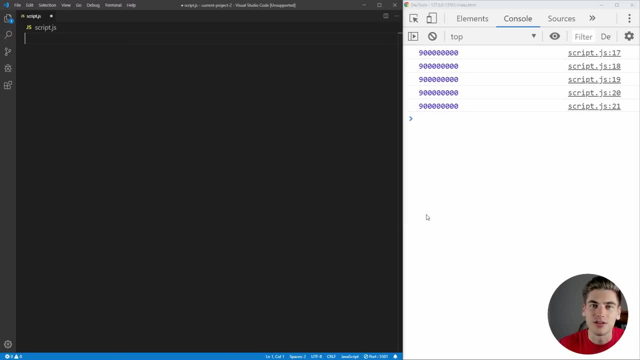 let's just remove all this code for now And imagine the Fibonacci sequence. If you know what the Fibonacci sequence is, essentially it just takes the previous two numbers, adds them together and that gives you the new number in the sequence. So we'll create a function called fib which takes 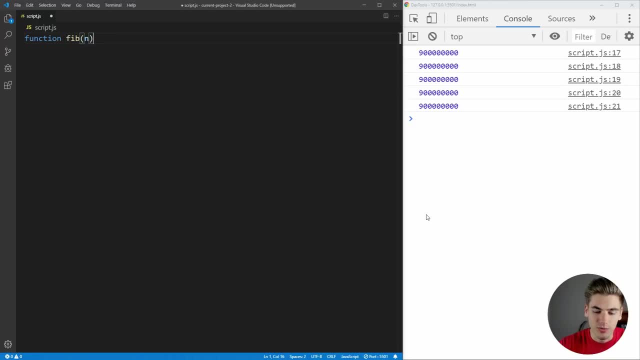 in n, which is the nth number of the Fibonacci sequence we want to get, And with the Fibonacci sequence, if n is either equal to one or two. so essentially we're going to say, if it's less than or equal to two, then we always are going to return one, because we need somewhere to start our. 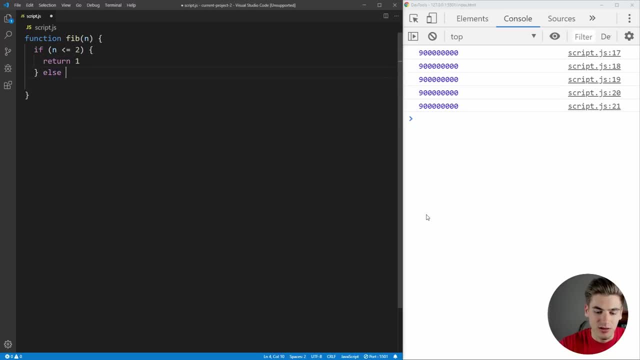 sequence. Otherwise, if it's not, we can just say here else then we can return the Fibonacci sequence of the previous number, just like this added to the Fibonacci of the second most previous number, so n minus two. And what we can do is we can just call this function and log it out. 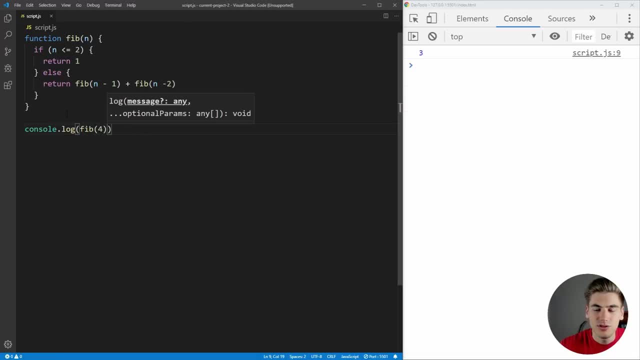 So we can say consolelog fib of four And, as you can see, we're getting three printed out, because the first number is one, second number is one, third number is two and the fourth number is three, two plus one. And this will work for all different numbers, for example six. But as we start, 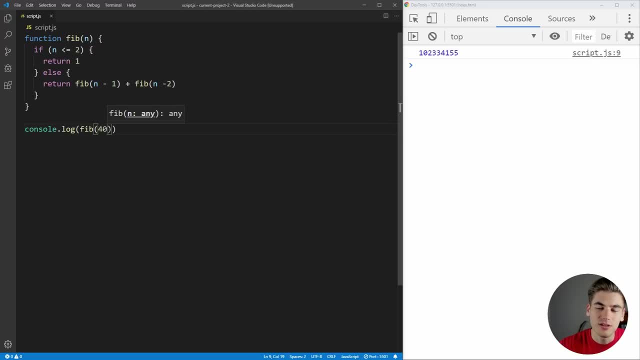 to increase the number. for example, if we go all the way up to 40, this is going to take quite a while. As you can see, it took maybe about a half a second to run, And as we get even more, let's just. 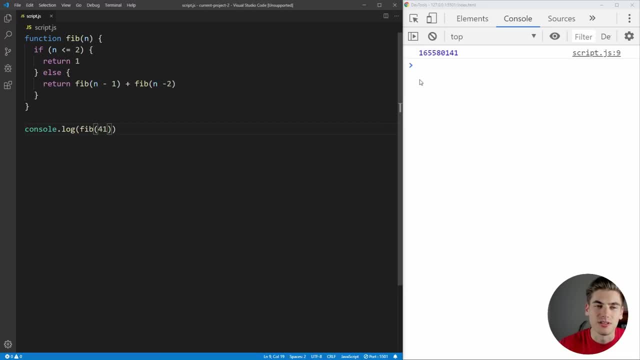 say 41, you can see it's taking even longer. that's close to double as long as 40 took. So it just gets slower and slower and slower, really quickly. But that's where memoization comes in. You see, with the Fibonacci sequence, when we are calculating these numbers, we're recalculating. 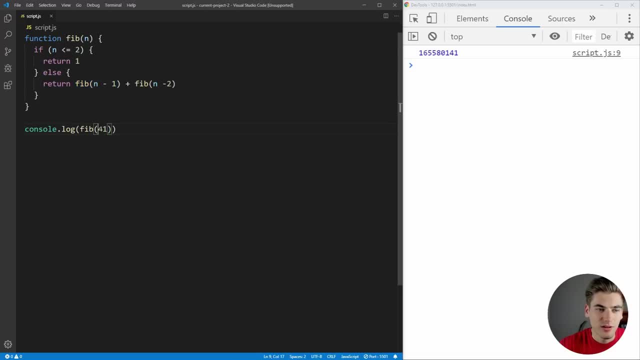 a bunch of the same things over and over again. For example, just to get the Fibonacci of number five, for example, we need to calculate the Fibonacci sequence of four right here and three right here. And then, in order to calculate four, we need to get the Fibonacci sequence of three and 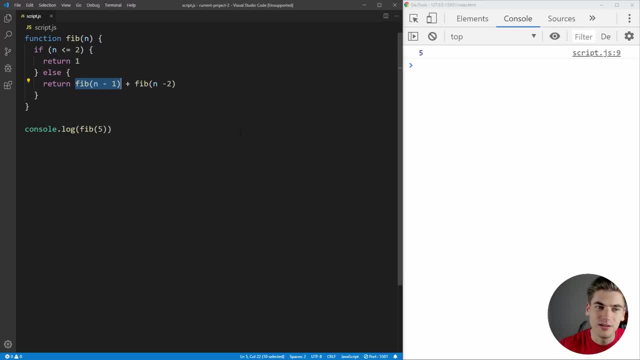 two. So right there, we've already repeated getting three Twice, And we also have to repeat two three times and so on. So we're repeating a bunch of these Fibonacci calls, which is where we can do memoization. So we can just come in here And we 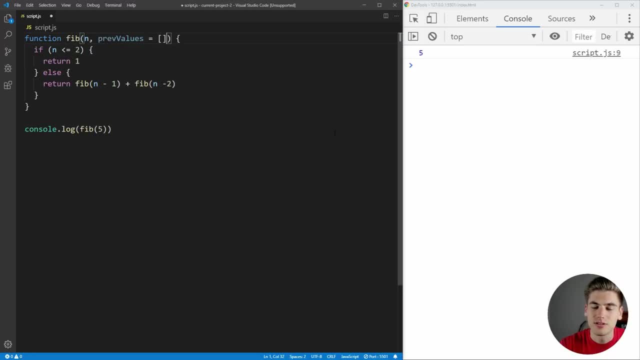 can say that we want to calculate our previous values And we'll default this to an empty array, So we can actually pass these previous values into our other Fibonacci sequences, saying: hey, we've already calculated this, you don't need to recalculate it. And then we just do a. 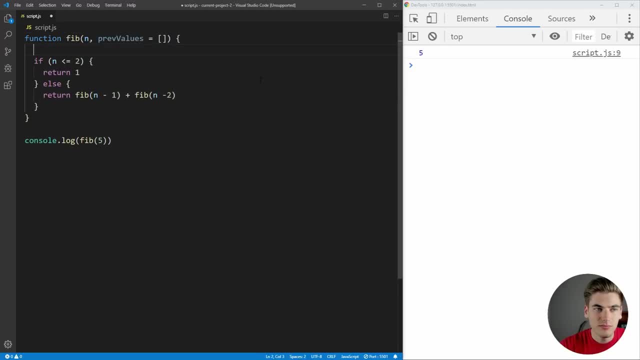 very similar thing to what we did with that square function. So the first thing we want to do is we're going to create a variable, we're going to call this our results, just like that, get rid of that equal, And then in here we just want to set our result equal to one if n is less than or equal to. 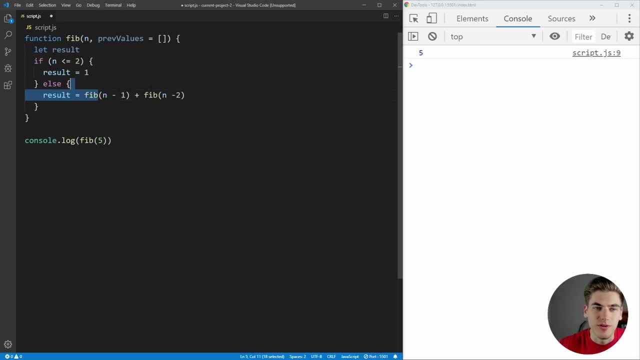 two, And here we're going to set our result equal to the fifth of n minus one plus the fifth of n minus two. Now what we can do is we can actually take our previous values of n And we can actually set this here equal to our result, just like we did in the previous example. And then, lastly, 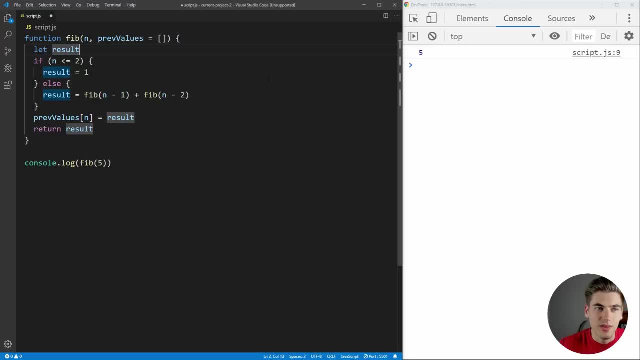 we just want to return our result At the bottom here, And then all we need to do is we just check for our previous value. So we say, if previous values of n is not equal to null, then we can just return the previous values of n. 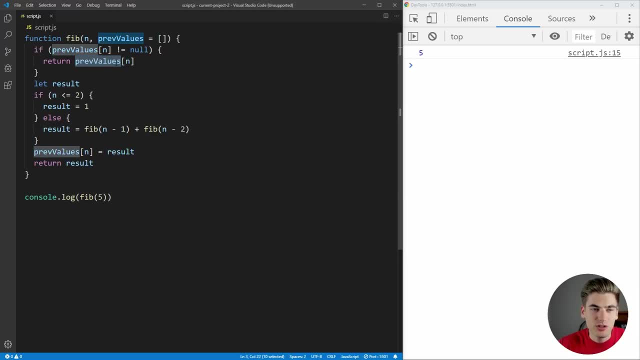 just like that. Now all that's left to do is to make sure we pass this previous value array down to all of our other calls of this Fibonacci function. just like that, And now they have access to the previous values from all of the other calls. 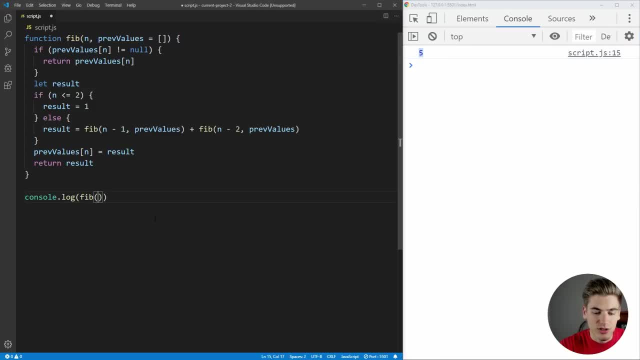 And if we say that you see, this is still working over here. But if we change this to be a large number, for example 40, you still see that executes almost instantly. What about 100?? Again it executes almost instantly. And with the other example, without memorization and without dynamic, 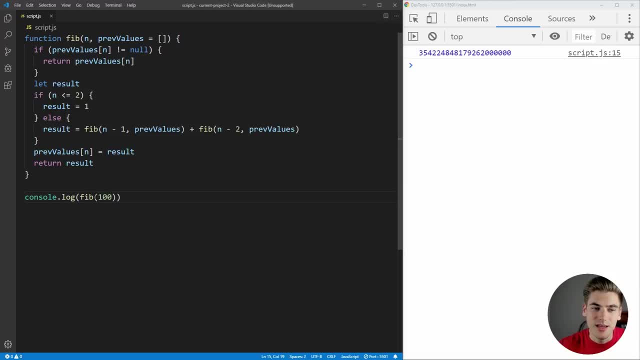 programming. it would have taken an incredibly long time to execute Fibonacci of 100. And we can even go further. For example, let's say we wanted to do 500. You can see that still is incredibly quick, especially compared to the old method. And that's all there is to memorization. 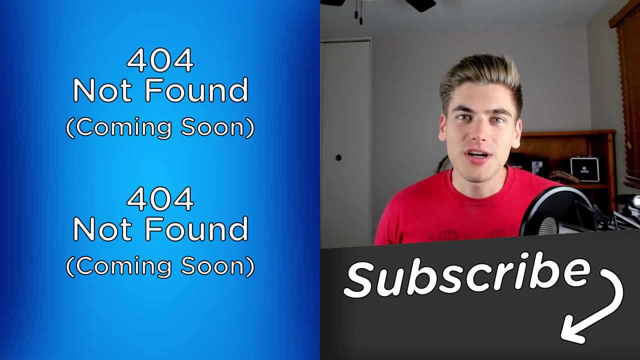 And dynamic programming. If you enjoyed the video, make sure to check out my other videos linked over here and subscribe to my channel for more videos just like this one. Thank you very much for watching and have a good day.